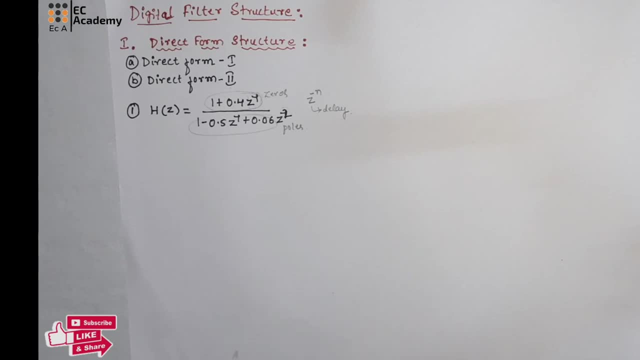 So z to the power of minus 3 will represent three step delay. likewise, Now let us represent this transfer function in direct form. 1. To represent any given transfer function in direct form: what you do first you write x of n. 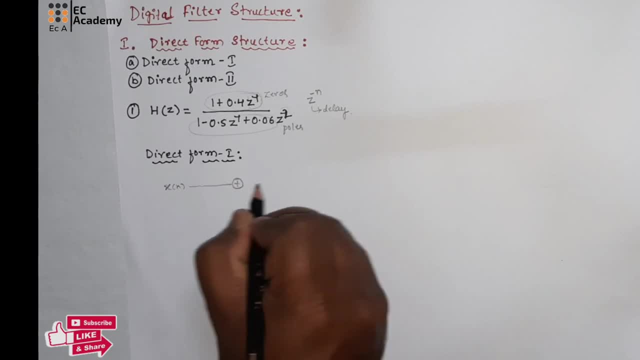 write a signal flow, write a summation, write one more summation and write y of n. This will be common for most of the problems. Always remember the direct form representation is nothing but the signal flow representation of the given transfer function. 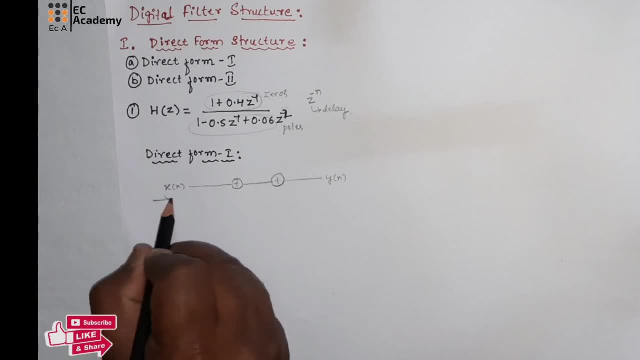 To write the signal flow: this side, we will write zeros, and towards this side, we will write poles. Okay, So, from this side, we will write zeros and towards this side, we will write poles. Now let us take the numerator, which represents the coefficient of zeros. 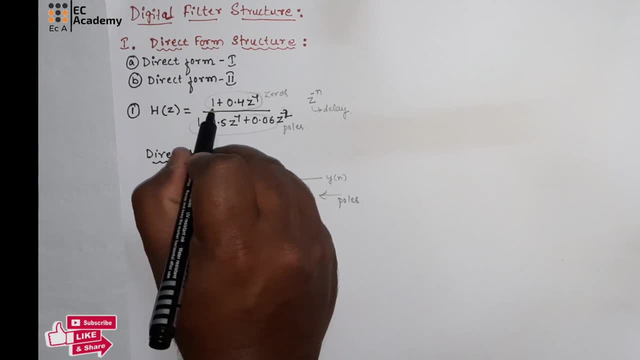 So here the numerator is given as 1 plus 0.4 z inverse. So what we can do, we can write x of n, here We will write a signal and here it will be 1.. So this is 1.. 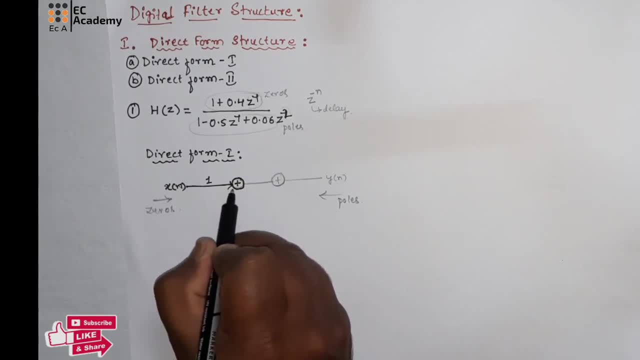 So we are having already a summation That represents plus. So we need to write a delay here. So we will write a delay that is z inverse and the coefficient is 0.4.. So we will write the coefficient here that is given to this summation. 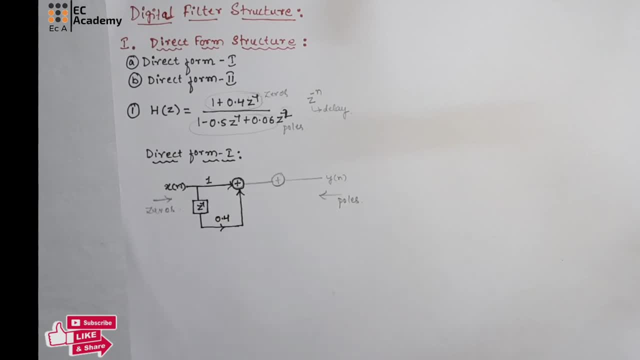 So the coefficient is 0.4.. So this is the numerator part that represents. So the denominator is the coefficients of poles, So here 1 minus 0.5.. So we will take the signal flow graph like this: 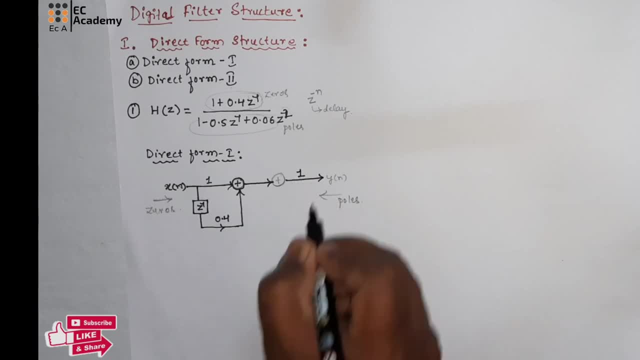 So this is given as 1.. So we will write summation itself. So we require one step delay, So we will take z inverse. So we will write z inverse. So the coefficient is 1.. So the coefficient is minus 0.5.. 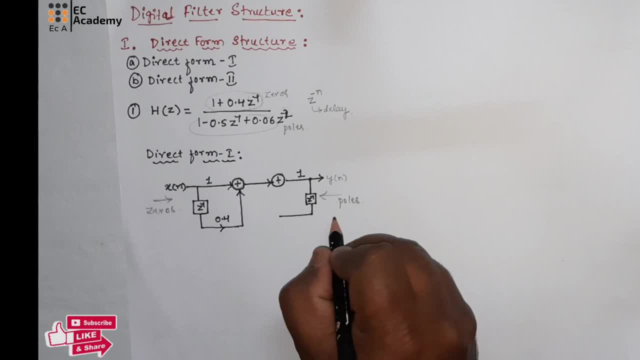 So here always remember while writing the poles: you will take negative coefficients of z inverse. So you will take always negative coefficients of z inverse. Which means, if you are having minus 0.5, you will take 0.5. 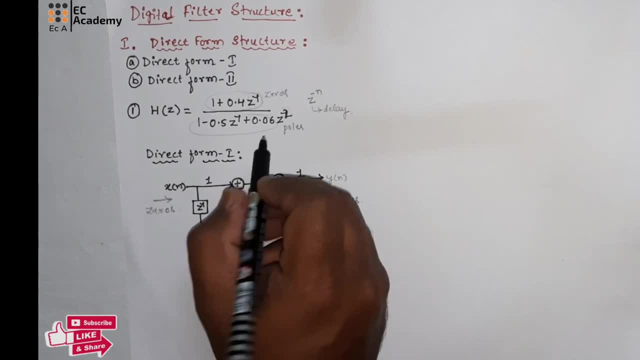 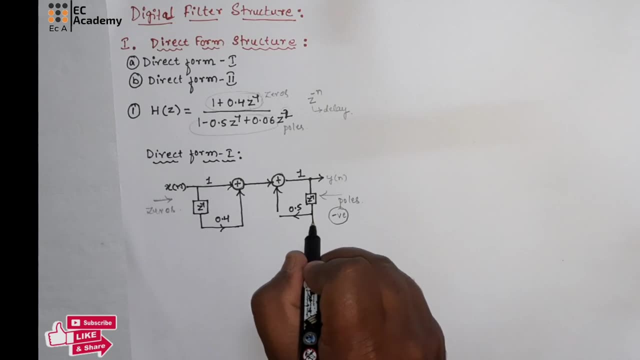 And that is given to this summation. So here we are having 0.06 with two step delay. So we are having one step delay here. For this we will add one more z inverse. That will make this as two step delay. 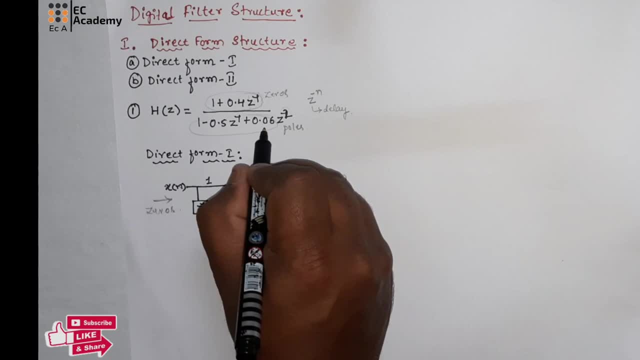 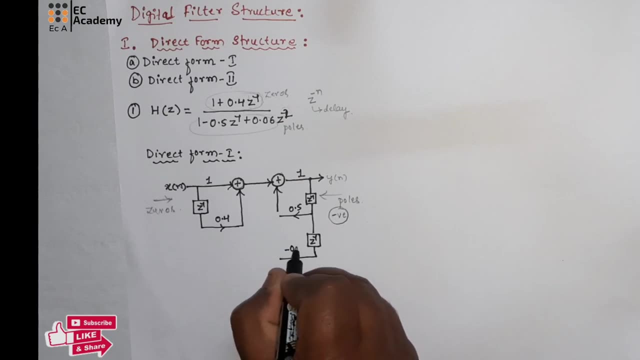 So for this the value is 0.06.. So we need to take the negative coefficients of poles, So we will write minus 0.06.. And here in between we are having the summation, So we will write one summation here. 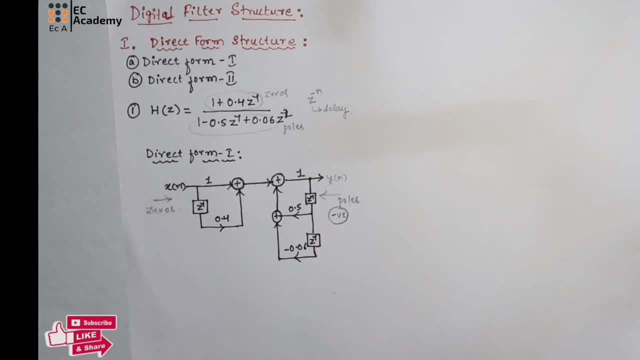 That is given to. So this is the direct form 1 structure of the digital filter. Now let us see the direct form 2 structure of digital filter. In direct form 2 structure, this end will write poles. You can see the arrow mark. 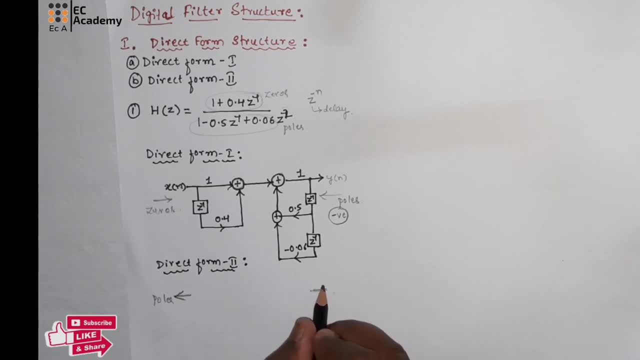 So it is towards left side And this end will write zeros. So here we will write poles, This end will write zeros, And instead of taking separate delay points for zeros and poles, we will take a common delay. Okay, The procedure will be similar. 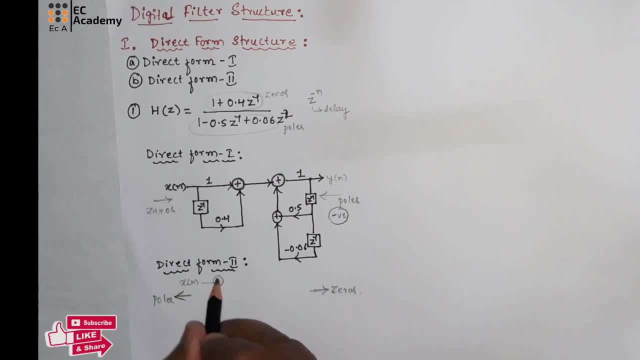 You can take x of n, You write a summation. Again, you write one more summation, You write y of n. So what we will do? Instead of taking separate delay, we will take common delay for Both zeros and poles in direct form. 2 structure. 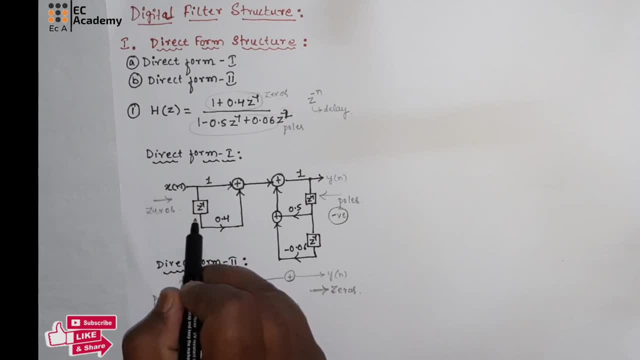 So here for zeros we require one step delay, For poles we require two delay points. So that is why generally we can take one delay plus one more delay. So we require two delay points So we can write x of n. 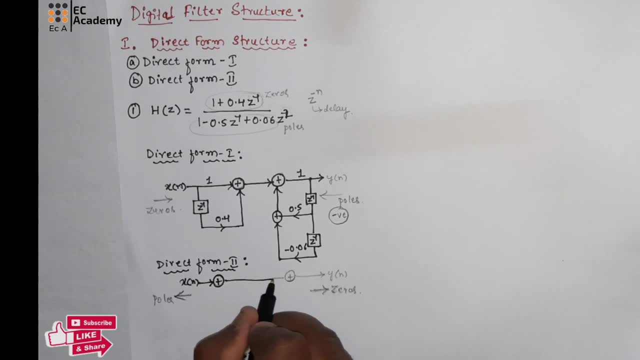 Summation, Again, one more summation, Again, one more summation. And here y of n. Here we will take two delay points, which is z inverse and z inverse. So at this end we need to write poles. 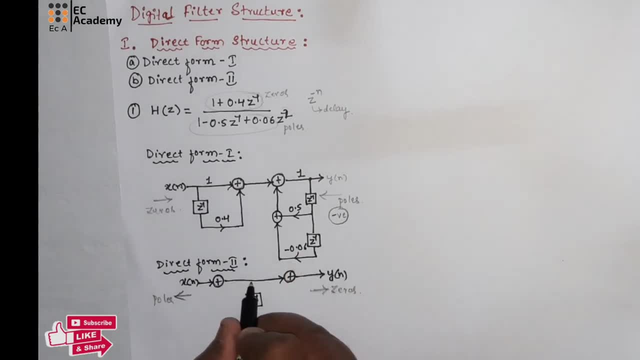 So we need to take this 0.5.. Again, we need to write poles. So we need to write negative coefficients for poles. So you add one more summation here which is given to this summation. So we need to write this coefficient. 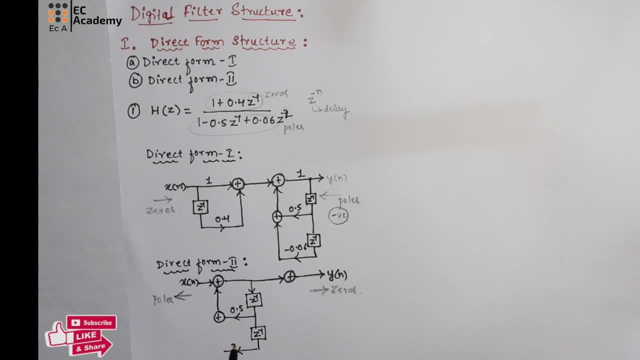 So it is minus 0.06 given to this summation And for zeros we are having 0.4.. So we can take from this end, which is 0.4, which is given to this summation. 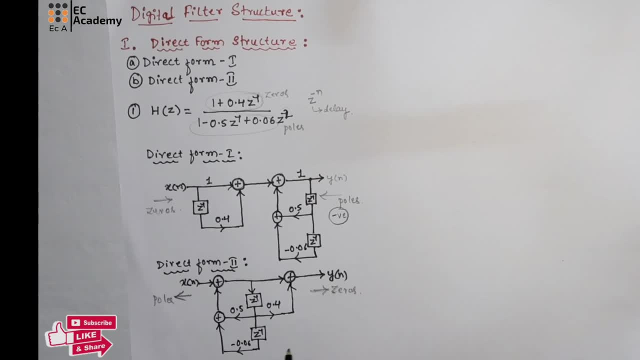 So this is the direct form 2 structure of digital filter. So here, if you observe, we are taking the common delay for both poles as well as zeros. Okay, So in direct form 2 representation, we are reducing the number of required delays. 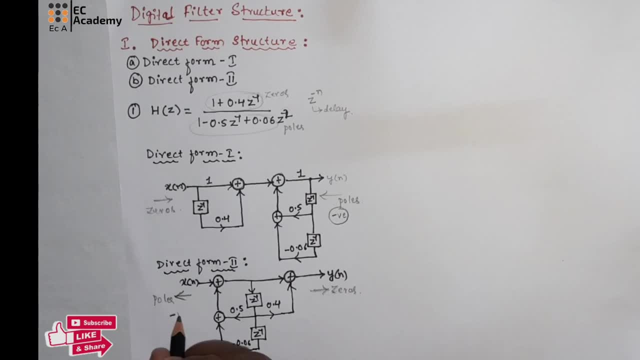 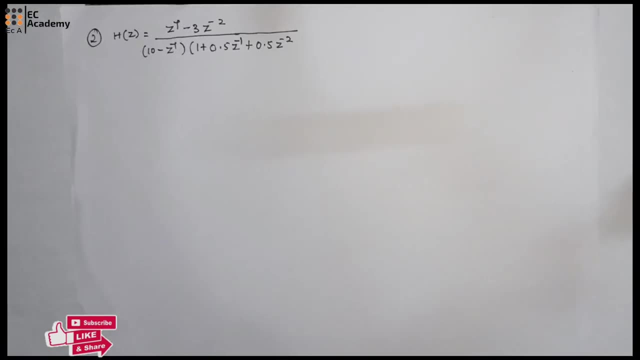 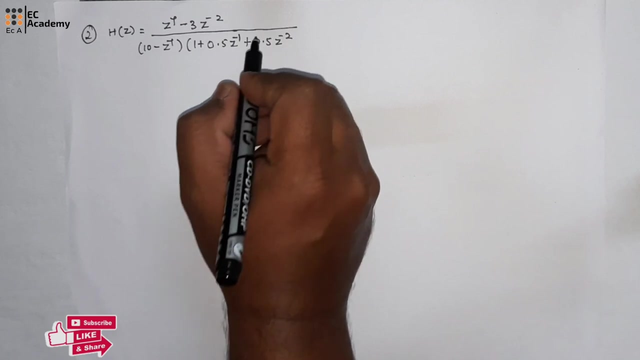 So always remember the coefficients of pole should be negative. We will take negative value of coefficient of poles. Now let us take the second problem, where the transfer function is given. For this transfer function we need to obtain direct form 1 and direct form 2 structure. 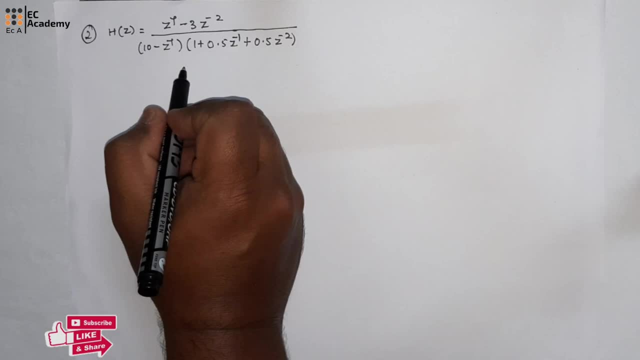 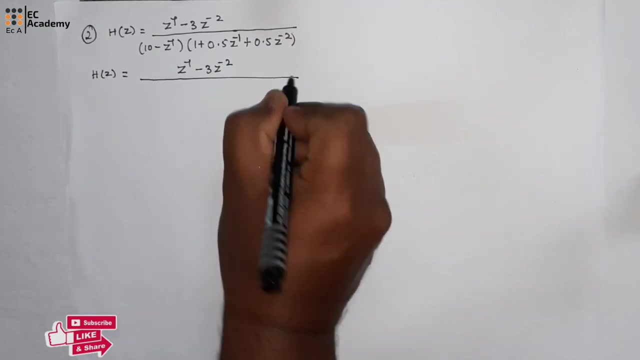 For this given transfer function. let us simplify before applying the direct form structure, So we can write the above transfer function: as h of z is equal to numerator, you write as it is z inverse minus 3, z to the power of minus 2 divided by: 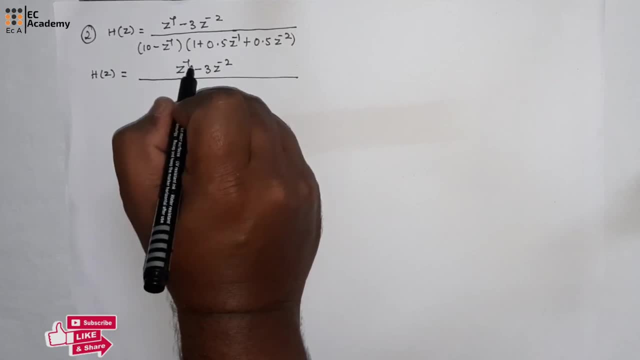 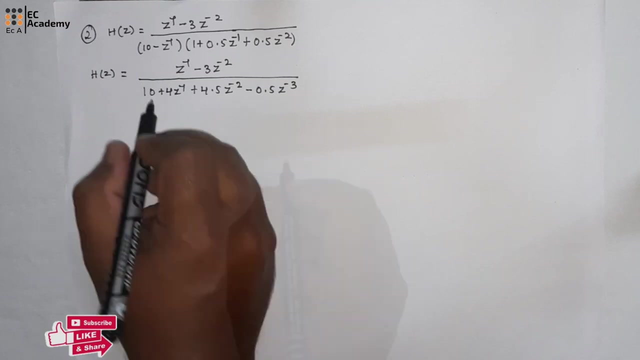 if you multiply these two terms in the denominator, you will get 10 plus 4 z. inverse plus 4.5 z to the power of minus 2, minus 0.5 z to the power of minus 3.. Here, always remember. 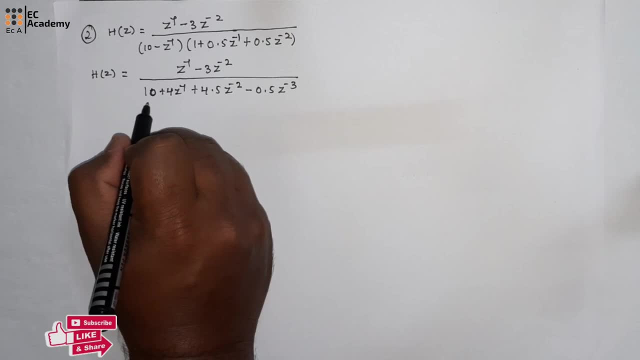 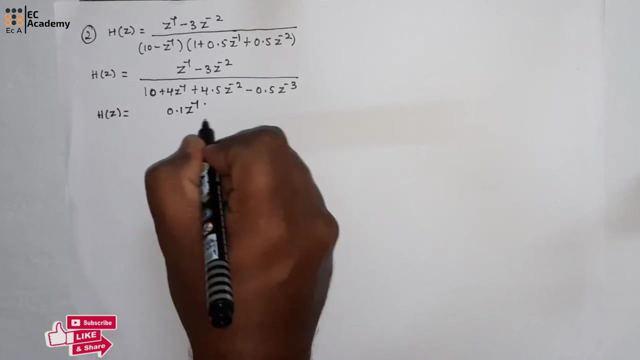 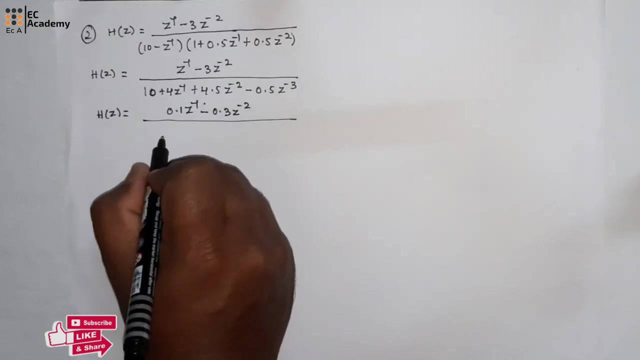 numerator or denominator. it should be in terms of y, 1 plus and the delay term. That's why we will divide numerator as well as denominator by 10.. So if we divide numerator and denominator by 10, so you will get 0.1 z inverse minus 0.3 z to the power of minus 2, divided by 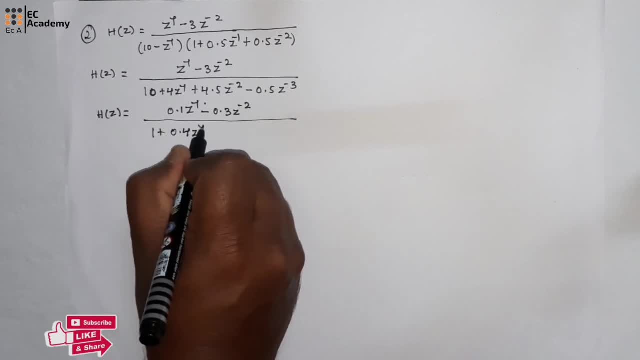 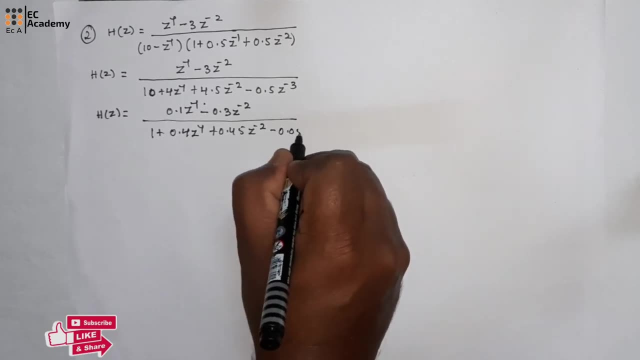 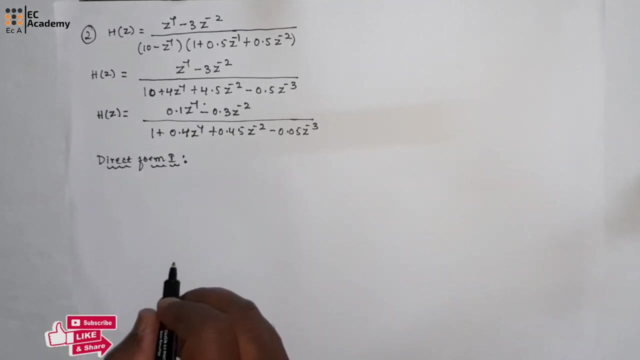 1 plus 0.4 z, inverse plus 0.45 z to the power of minus 2 minus 3.. So here, this is the numerator term, which represents zeros, and the denominator coefficients represents the poles. Now, first let us implement direct form 1 structure. 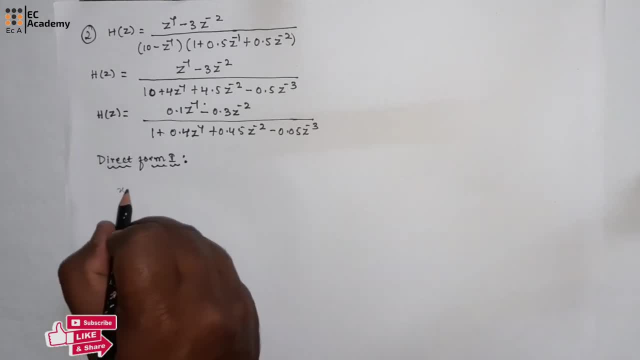 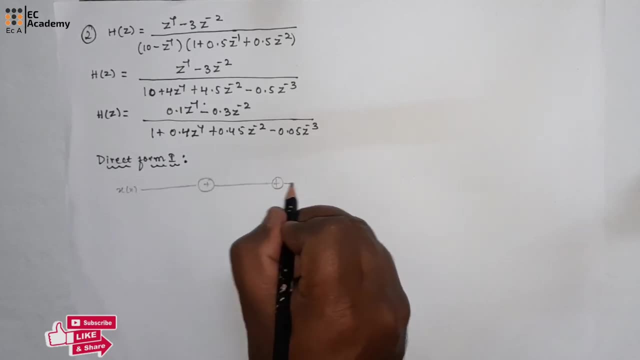 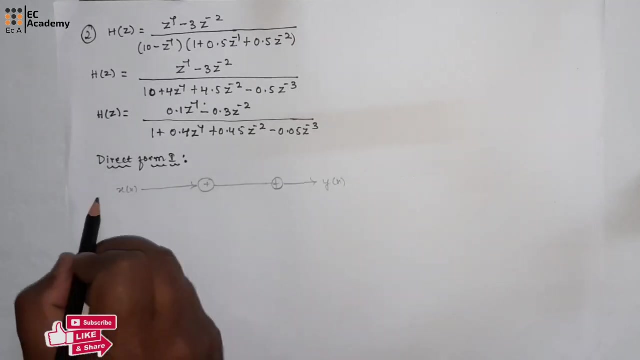 So, generally, you need to write x of n, with a summation here and one more summation, and y of n. Okay, so this is the numerator. so this is the first step which you need to write. so this end, you need to write zeros in this end. 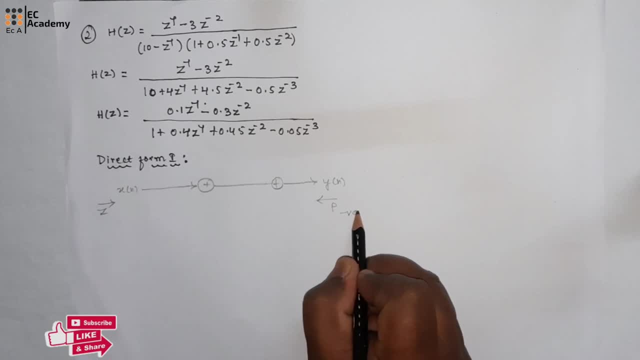 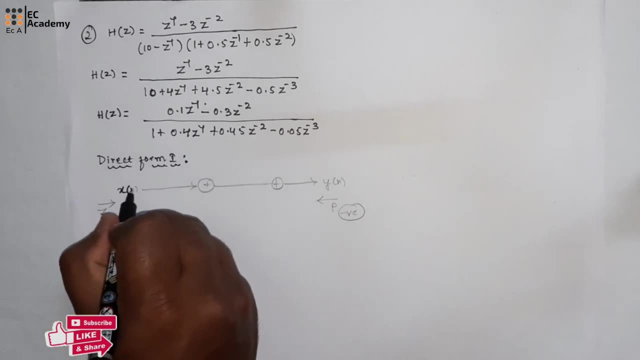 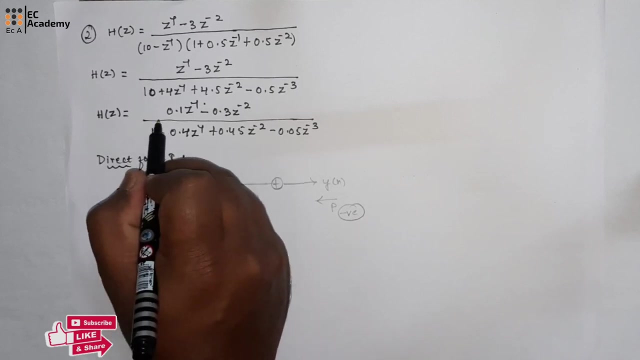 you need to write poles with negative coefficients. you need to remember this step. so x of n in the numerator you can observe there is no one plus term, right? so that's why, directly, you need to write this delay term. so from here we can take the delay term, which is z, inverse the coefficient. 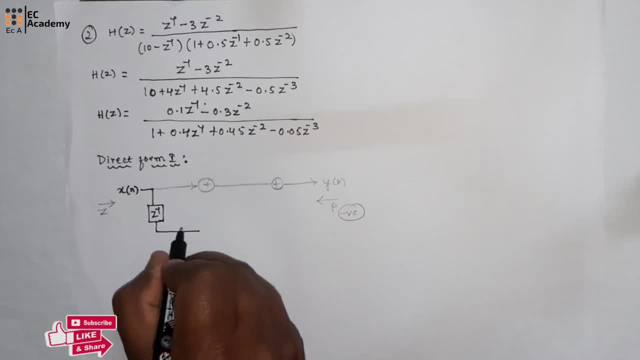 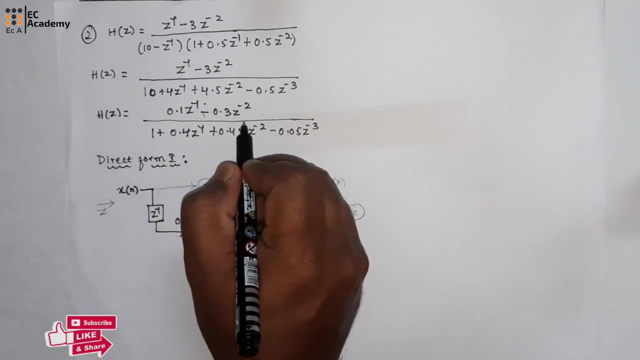 of z inverse is 0.1, so you write 0.1 and the second term is minus 0.3 z to the power of minus 2, which is two step delay. already there is one delay here. you can add one more delay, which is: 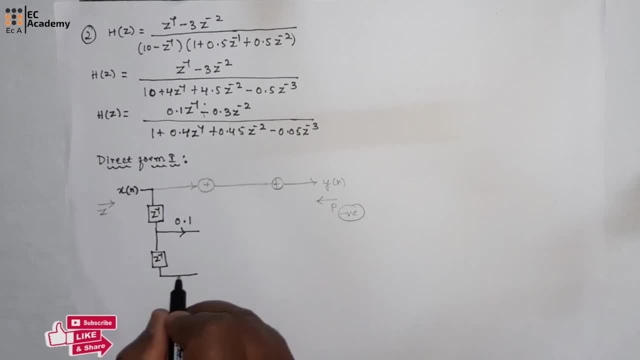 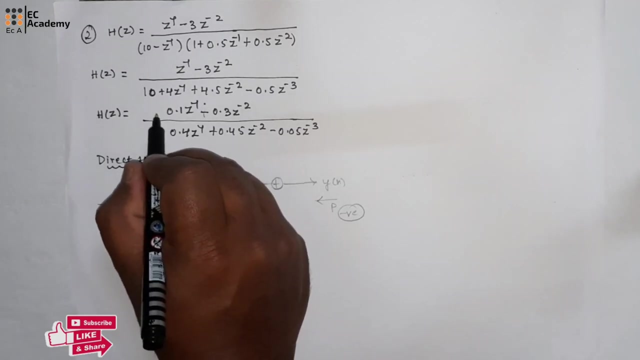 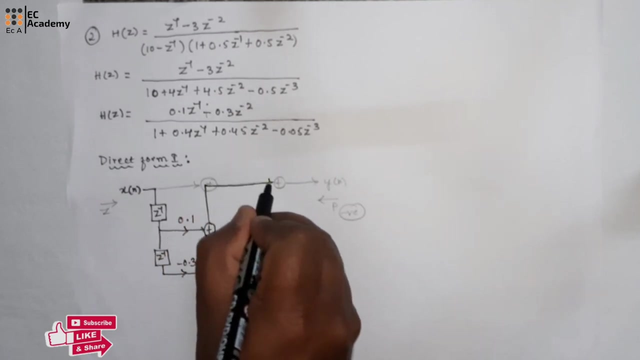 z inverse, here we will write minus 0.3. so here we can write a summation and you can write here. so here what we need to do, since we don't have any term before this delay, so we will not take this summation. we can directly write the arrow mark towards this summation. so 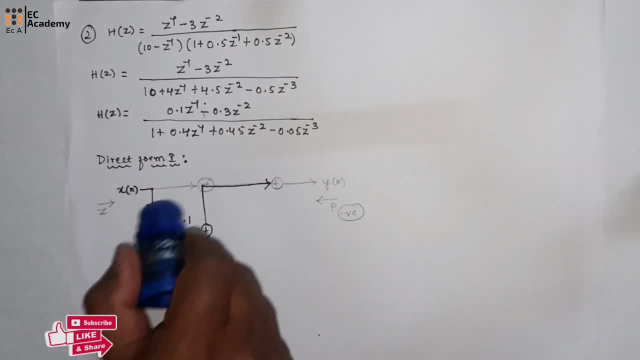 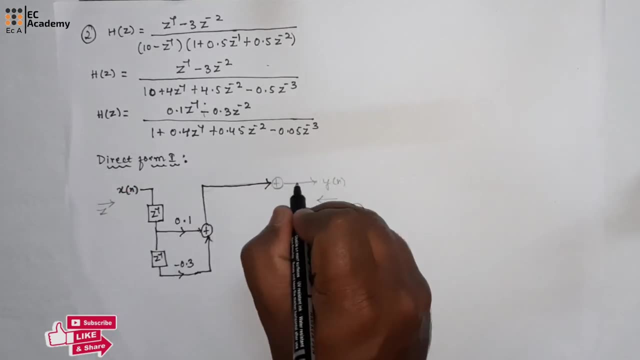 here, since we don't have any term before the delay, we will not take this signal flow here in the denominator we are having one, so you can write a summation. here you can write y of n, here you can write one. so here the first coefficient is 0.4, with one step delay. 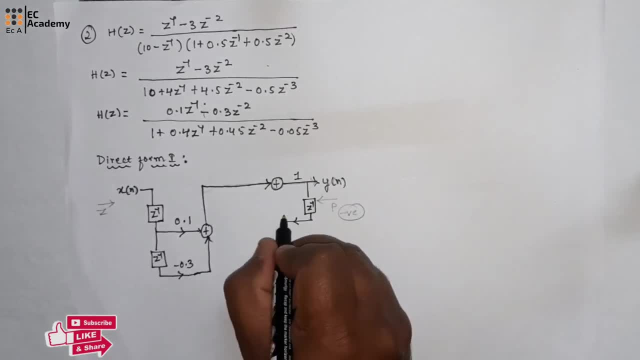 so it is. we need to take negative coefficients, so we'll write minus 0.4. so we'll take the second coefficient with two step delay and we'll write the negative coefficient of that one, so it will be minus 0.45. we'll take one more delay here. that represents total of three step delay. so the coefficient is: 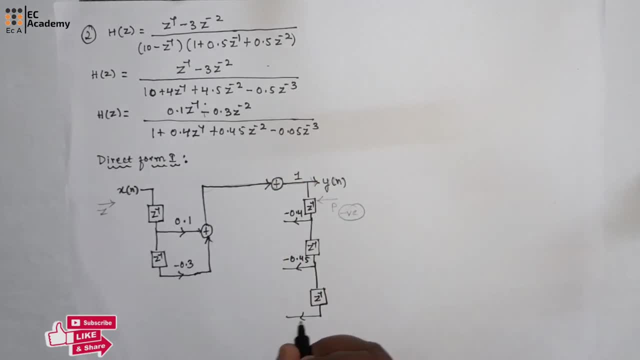 minus 0.05. for that we need to write 0.05. so you can take one summation here, one more summation and you can join the lines. so this is the direct form, one representation of the given transfer function. now let us see the direct form to representation of this transfer function. so this end we need to write poles, and. 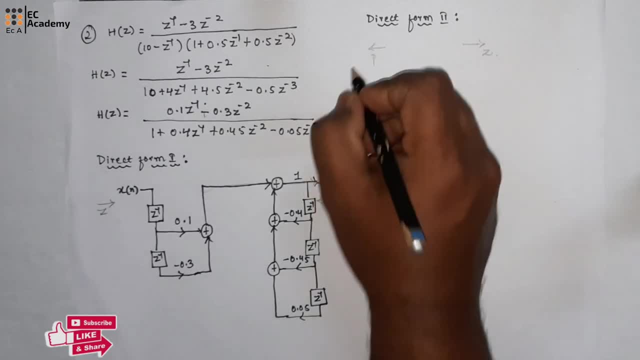 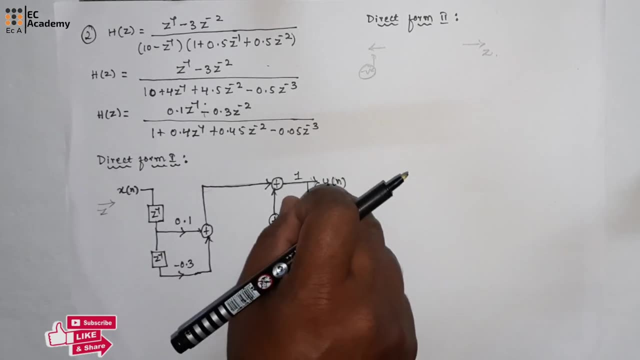 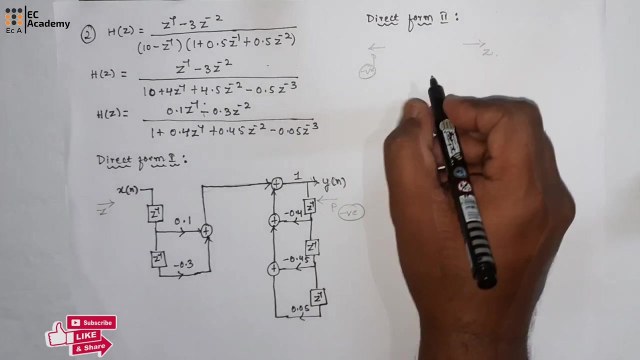 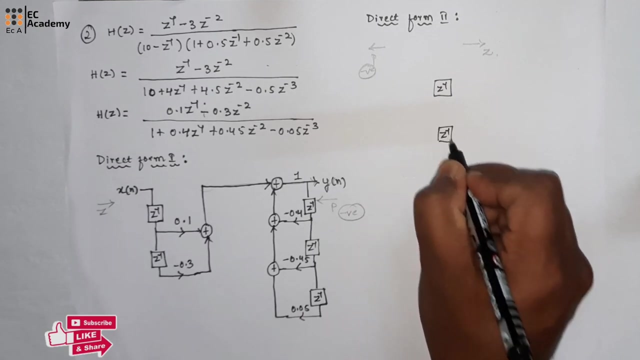 here we need to write zeros, okay, so poles with negative coefficient. so we need to take common delay in direct form. two structure, so we require three delays for poles, two delay for zeros. so we will take three delays in common, so we can take z inverse, z inverse and one more delay which is z inverse. we can write x of n. 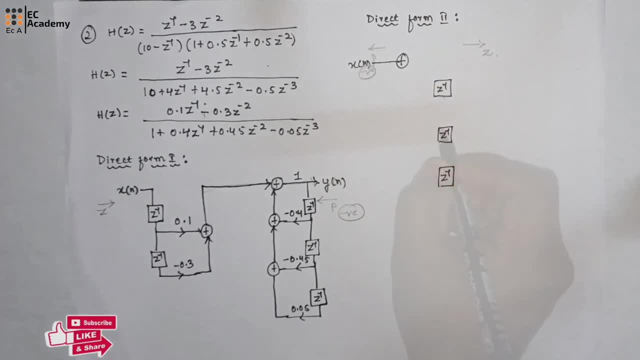 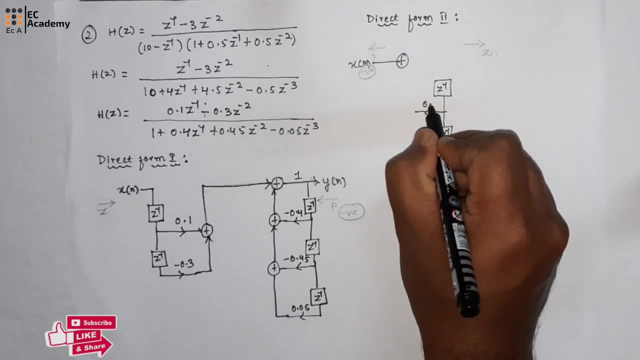 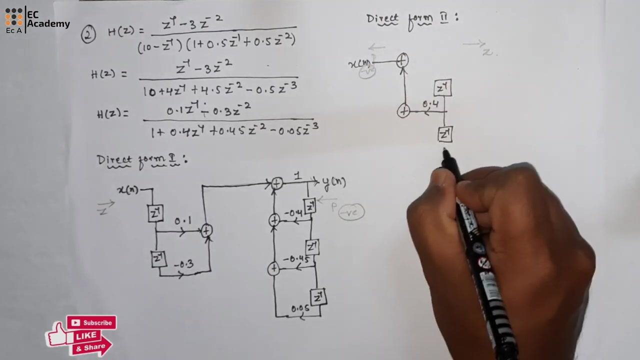 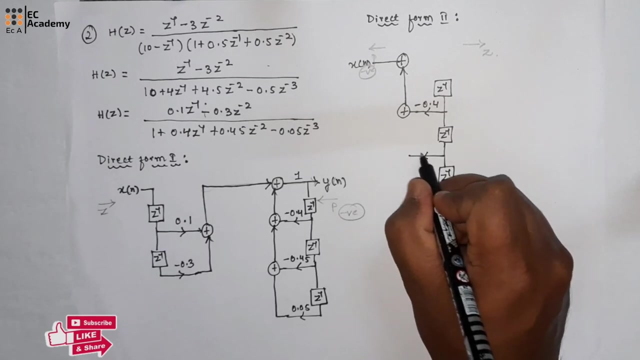 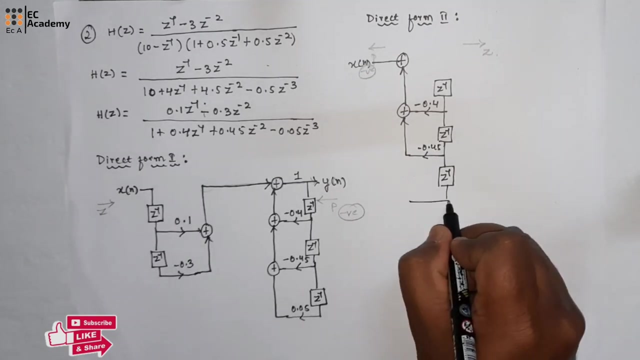 here with a summation. we'll write poles at this point, so we'll write the same structure, which is zero point four. so here it will be minus zero point four. so here it will be minus zero point four, five, and it will be zero point zero 5. so here it. 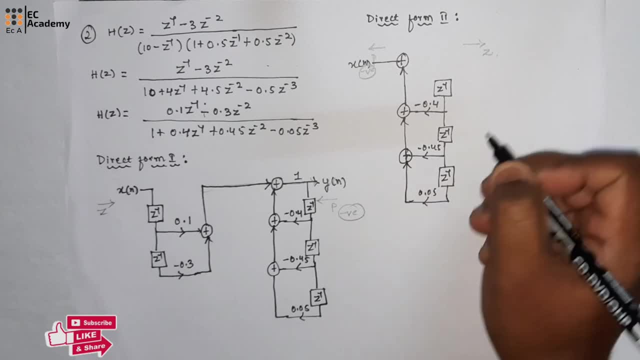 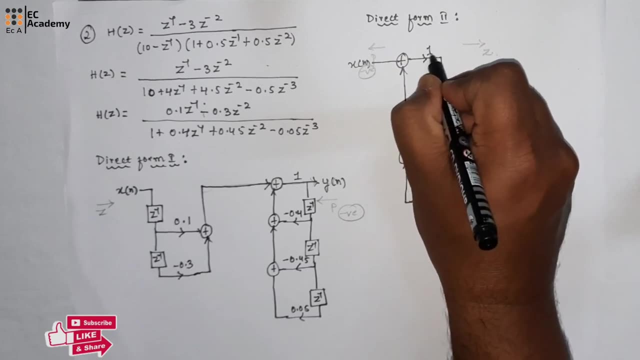 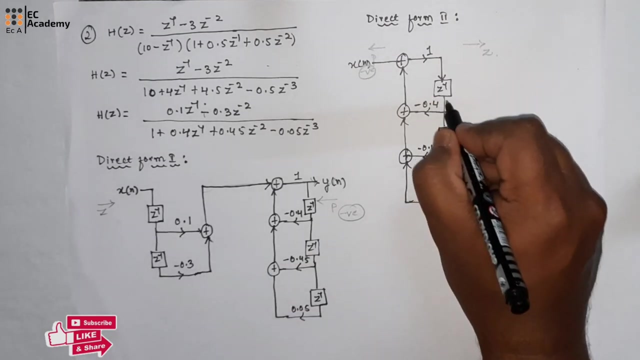 will be summation. so this value of 1 we will write here. so for 0 we require one delay. after one delay it will be 0.1. so after one delay it will be 0.1 and after two delay it will be 0.3. so you can write. 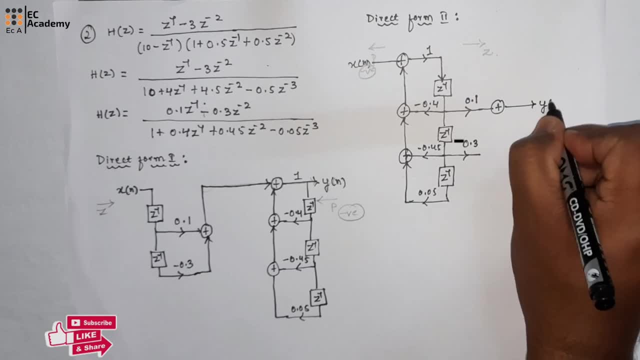 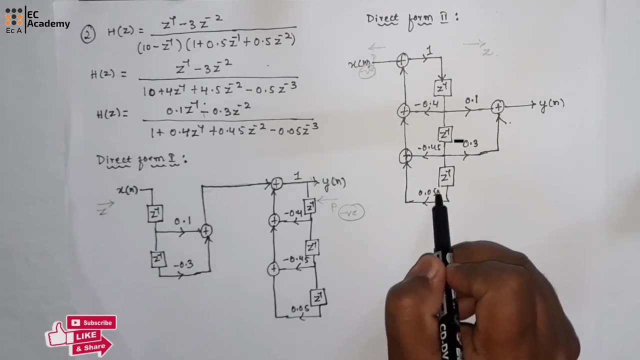 one summation here and you can write Y of n. so this is the direct form to representation of the given transfer function. sometimes in exam they will give the equation like this: for this what we need to do: you need to take Z, transform on both LHS as well as RHS. you need to take 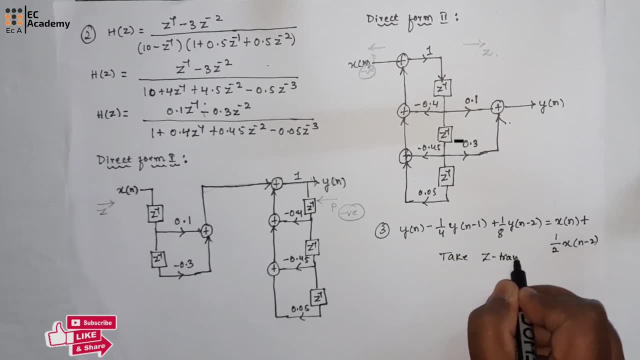 Z transform in both LHS as well as RHS. If you take Z-transform, you will get Y of Z minus 1 by 4 Z. inverse Y of Z plus 1 by 8 Z to the power of minus 2 Y of Z is equal to X of Z plus 1 by 2. 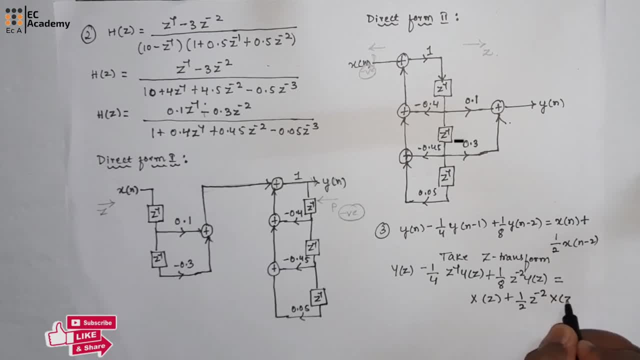 Z to the power of minus 2 X of Z. So in these two equations, if you take Y of Z and X of Z common and if you take the ratio Y of Z divided by X of Z, it will be equal to 1 plus 1 by 2 Z to the. 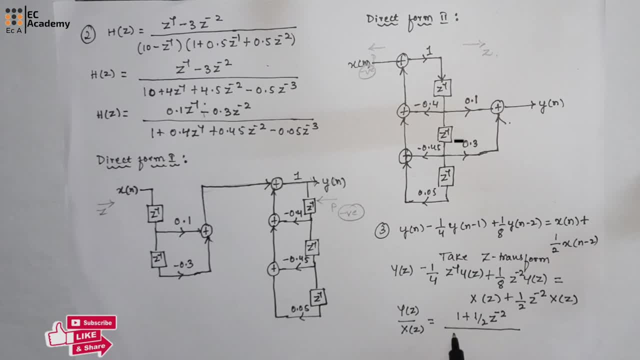 power of minus 2 divided by 1 minus 1 by 4 Z, inverse plus 1 by 8 Z to the power of minus 2.. So here, Y of Z divided by X of Z is nothing but H of Z. So for this function you need to: 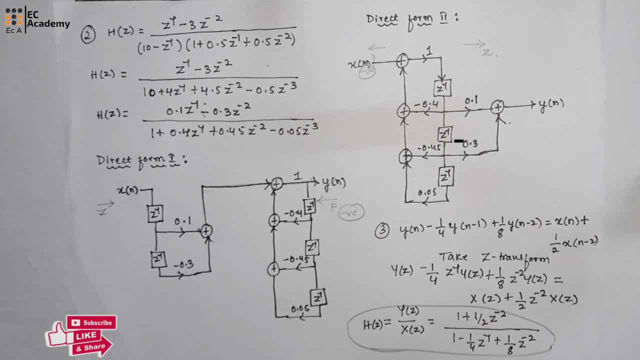 apply the direct form 1 and direct form 2 structure. So sometimes in exam they will give in this form. you need to convert this into the ratio of Y of Z divided by X of Z to get H of Z. So this is about the problem on direct form structure of. 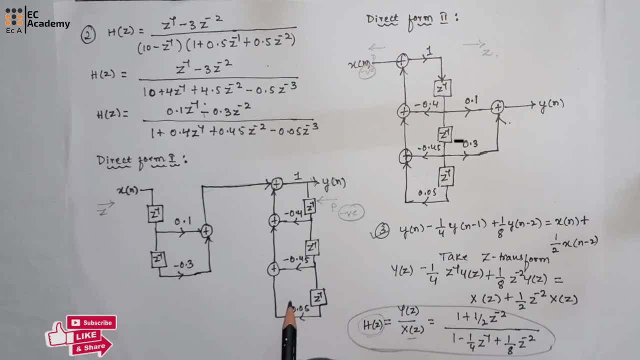 the digital filters. Hope you have understood the topic. Thank you.